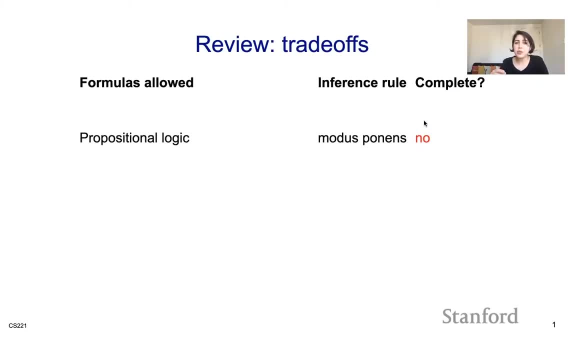 and the idea of an inference rule is: can we do a manipulation of syntax in the syntactic land over formulas in order to derive, in order to prove a new formula? And the idea is: is that inference rule under that specific set of logic, illogical formulas? is that sound and 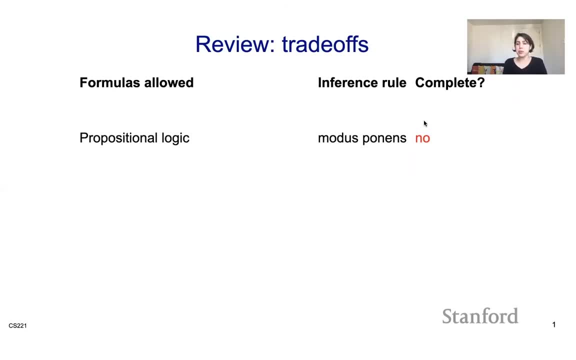 complete. And what we have seen is, if I apply just modus ponens on propositional logic, I get soundness but I don't get completeness. And then what that means is if I have a bunch of formulas that are entailed, that are true, I'm not going to be able to get all of them. if I 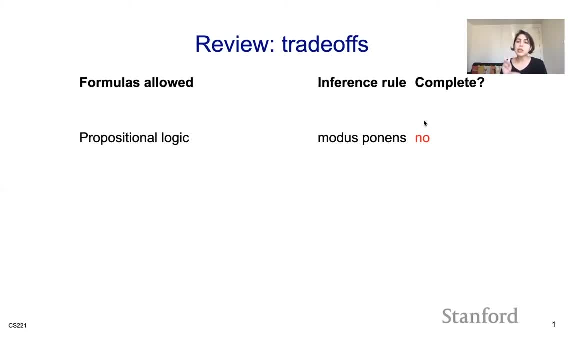 apply modus ponens on propositional logic. So we talked about two ways of solving that and we discussed the first way. The first idea was, instead of looking at all of propositional logic, let's look at a subset of it, and that subset is propositional. 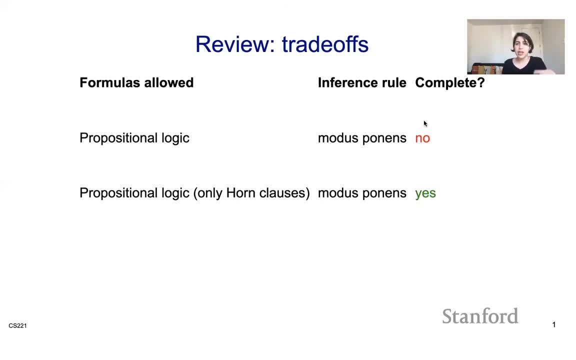 logic with only horn clauses. So we defined horn clauses during the last module and we looked at propositional logic with only horn clauses and in that case if I apply modus ponens, then I get soundness and completeness. everything is great. The other option is: what if I don't? 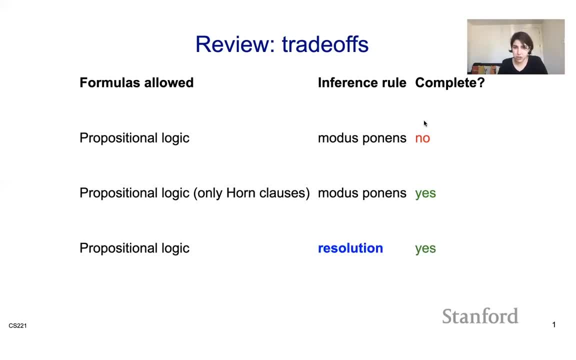 want to limit my propositional logic. What if I want to look at all of propositional logic? can I make my inference rule a little bit fancier, a little bit more powerful? So in this module we are going to be talking about a new type of inference rule, specifically, 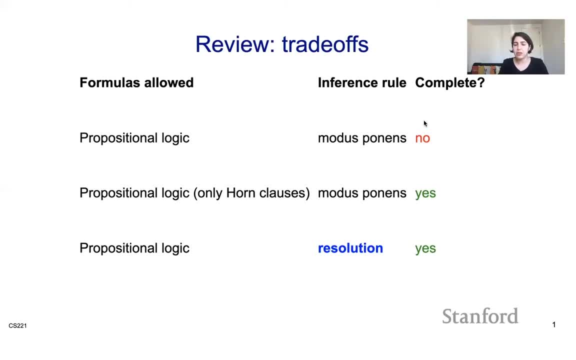 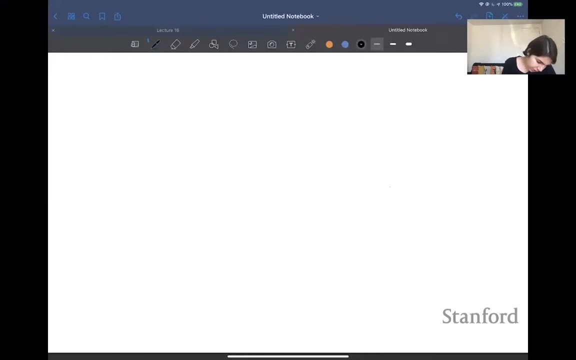 called resolution, as a way of getting both soundness and completeness. All right, so to start with, I want to just write out a few things that we're all aware of, but let's just get on the same page on all of them, So all right. so let me just write out a few things. So, if we have p implies q. 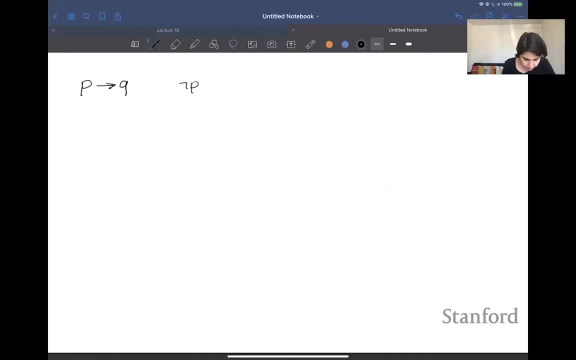 what is that equivalent to? That is equivalent to negation of p or q. Let's just write out some of these equivalences here. If I have negation of p and q, what is that equivalent to? Well, I can apply De Morgan's law and that gets me negation of p or negation of q. And then, if I 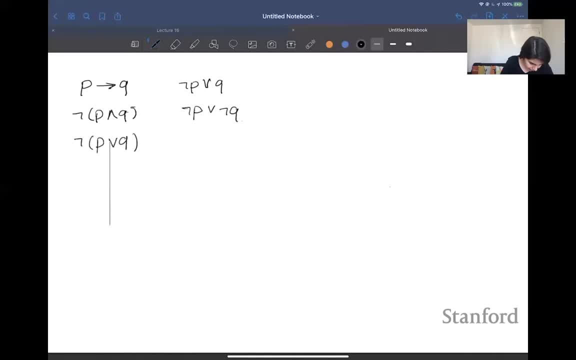 have negation of p or q, what is that equivalent to? Well, I can apply De Morgan's law and that gets me negation of p or negation of q. And then, if I have negation of p or negation of q, what is? 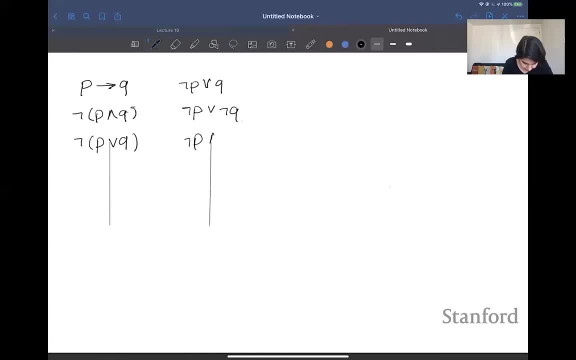 that going to be. That is going to be equal to negation of p and negation of q. All right, so these are a few equivalences that we all agree over. This is just how they are. It's just like truth, right. So if you look at the truth table of these, you're going to get these equivalences. 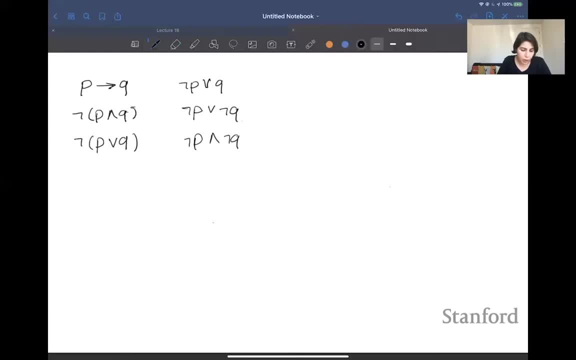 And the reason I'm defining these equivalences is: in general, I would like to write everything in the form of disjunctions and conjunctions, So let me define a few other things here. So I'm going to define a literal as a propositional symbol, p or a negation of a. 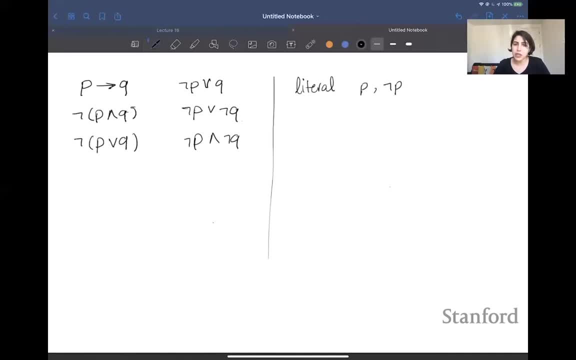 propositional symbol. negation of p- So a literal is just p. or negation of p, where p is just a propositional symbol. So then, based on that, one can define a clause to be a conjunction- sorry, to be a disjunction- of a propositional symbol. So I'm going to define a literal as a. 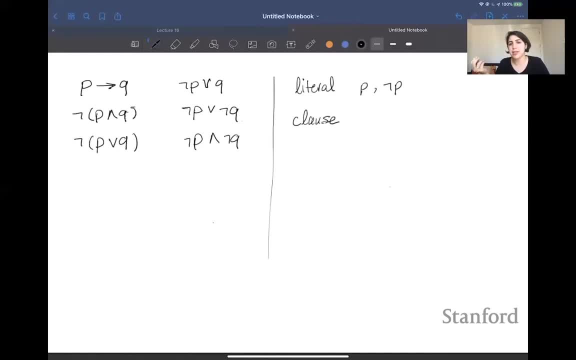 propositional symbol. So we talked about horn clauses during the last module but we never defined what a clause is. So a clause is just an or of a bunch of literals, It's just a disjunction of a bunch of literals. So I can have a clause that's like p1, or negation of p2, maybe, or p3.. 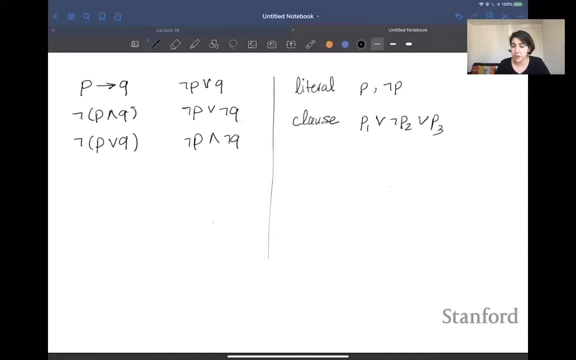 This is a clause because it's just an or of a bunch of literals. So then the question is: what is a horn clause? So could we? we defined horn clauses last lecture, but we could think of horn clauses a little bit differently here. So a horn clause is basically a clause, it's just a. 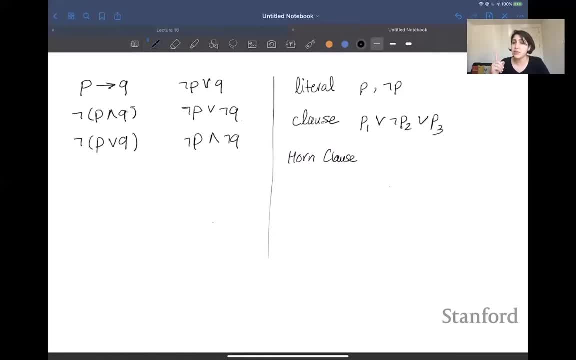 disjunction of a bunch of literals with at most one positive literal. So I'm going to refer to this guy as a positive literal and this guy as a negative literal. And a horn clause basically says: you have at most one positive literal in your clause. For example, this clause that I've written: 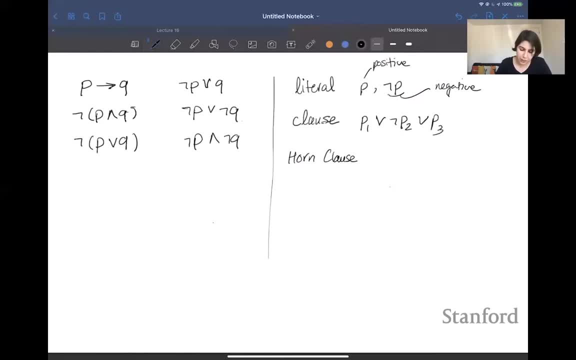 here is not a horn clause right, Because it has two positive literals, p1 and p2.. So it's just a p3.. But, for example, I can have another horn clause that is p1, or negation of p2, or negation of p3. 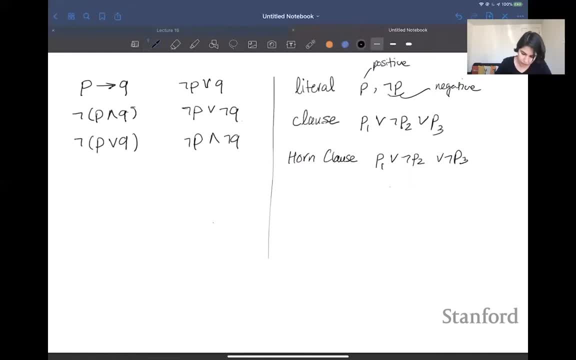 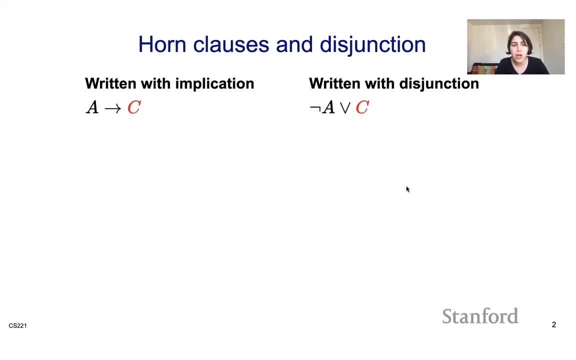 And then this is going to be a horn clause because it has at most one positive literal, that that is p1. So this is just another way we can get horn clauses. So going back here, right, so we have a implies c. How can we write it? We can write it as negation of a or c. We have a. 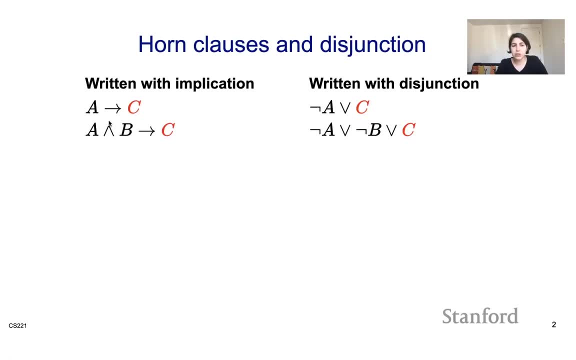 b implying c. right, What is that? equal to It's negation of this first part. I can use the Morgan's law and that gives me negation of a or negation of b or c. Remember, like again, this is a clause. 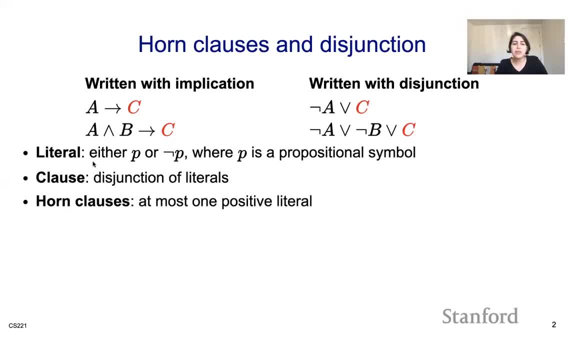 now, and it's a horn clause, And again, like defining what I've defined so far, a literal is going to be a prepositional symbol, either positive or negative, either p or negation of p. A clause is just a disjunction of these literals And a horn clause is just a clause with at most one positive. 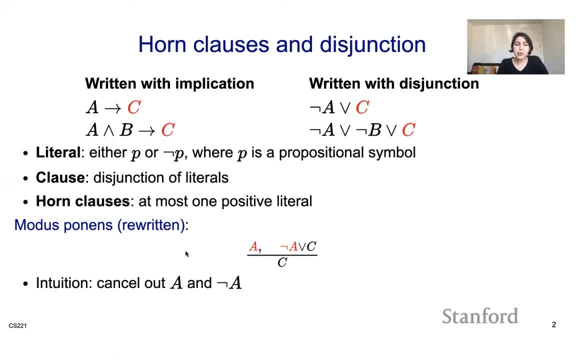 Okay, All right. So now when I'm thinking about modus ponens, I can actually write it out as clauses, right? Like, remember, I have a and a implies c and that gets me c. That is what modus ponens tells me. Instead of a implies c, I can just write it as a clause and I can write: 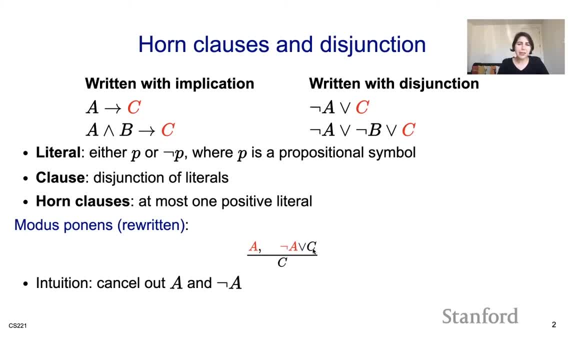 it as negation of a or c, okay, And kind of like, intuitively, like what is really happening is you're canceling out a and negation of a. That's why you're getting c okay. And the reason I'm defining modus ponens like this- I'm rewriting it- is this kind of helps. 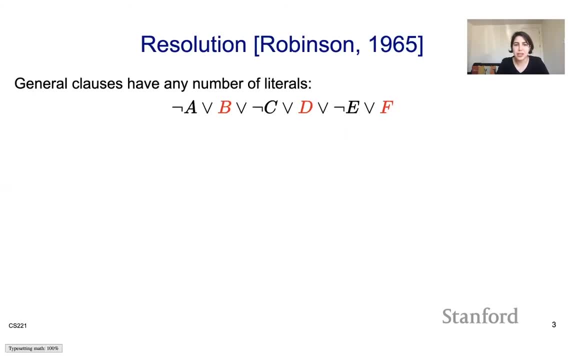 us to think about this more general resolution rule that I'll be talking about in a few slides. Okay, So the idea of resolution is: I don't want to limit myself to specific types of clauses. I can talk about general clauses, And general clauses are, what are they? They are disjunctions. 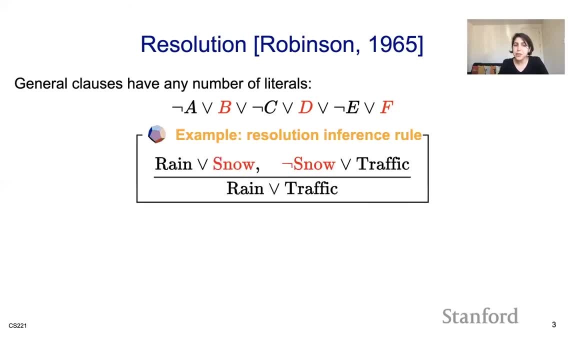 of positive or negative literals, And the idea of resolution is: if you have a bunch of clauses, you will have a rule. you will have an inference rule that cancels out your positive and negative literals. So here is an example. So if it is raining or snowing, that's part of your knowledge. 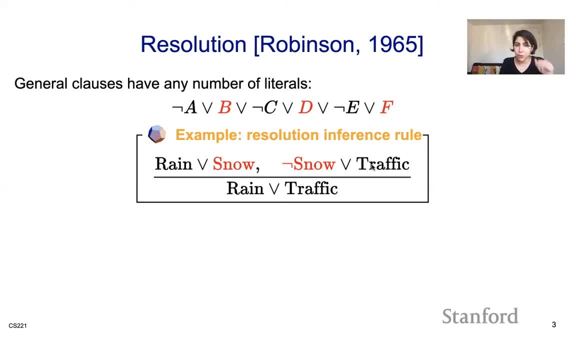 base and if it is not snowing or there is traffic, one can infer that it is raining or there is traffic. Let's think about like: why can't we, why can we infer this, even intuitively? okay, So if it is snowing right, So if it is snowing right, So if it is snowing right, So if it is, 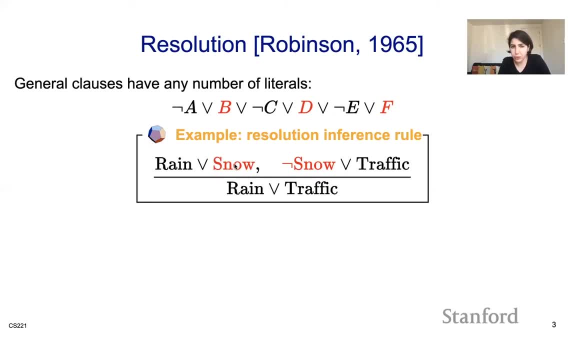 snowing, then there has got to be. if the snowing is true, right, There has got to be traffic. okay, So that's how I get traffic. And if it is not snowing, right, If it's not snowing, then there. 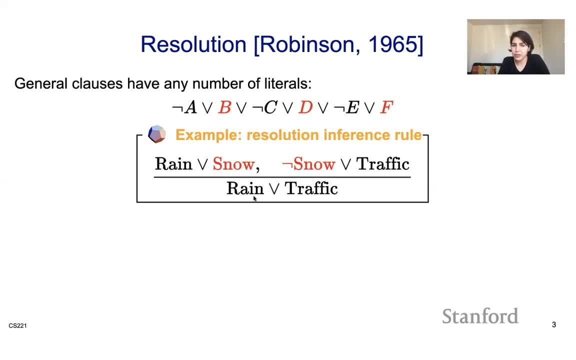 has got to be raining, because it's either snowing or raining. So that's how I get rain, So intuitively. that is why you're getting this rain or traffic And in some sense you can think about snow and negation of snow cancelling each other out, because either if it is snowing or if it is not snowing, 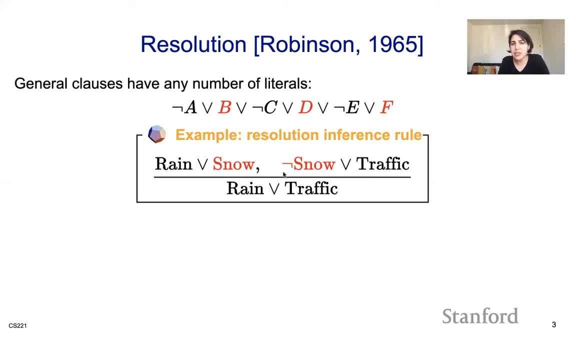 we are going to get traffic or rain out of it, And then this is basically resolution. inference rule applied to one example. okay, One can think about this much more generally and think about a clause f1 or disjuncted through fn or p, and then another clause where you have negation of p. 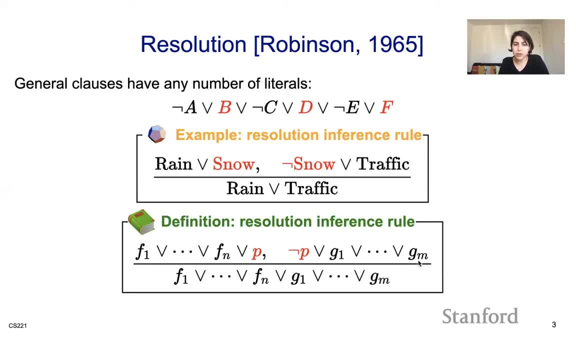 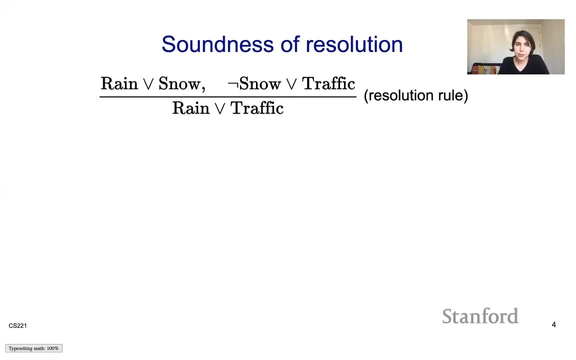 or g1 through gn, And then the idea of an inference rule is based on these two premises, we can conclude a new clause that cancels out p and negation. Okay, So this is called resolution. All right, So is resolution sound? So that's a very good question to ask. In general, we want it to be. 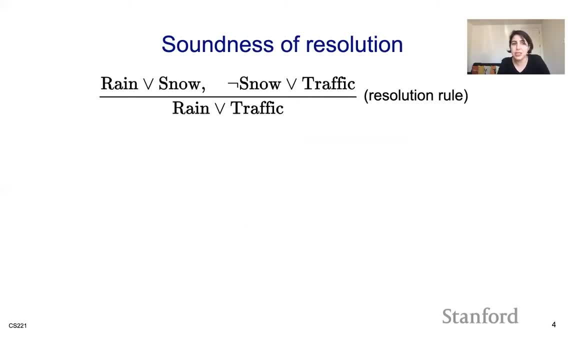 sound, because we want to be able to derive things that are actually true. So is it like- remember this example- is it true that I can derive rain or traffic here? Okay, So how do I check that? Well, to check soundness, I need to actually get to the models and meanings of each one of these formulas. 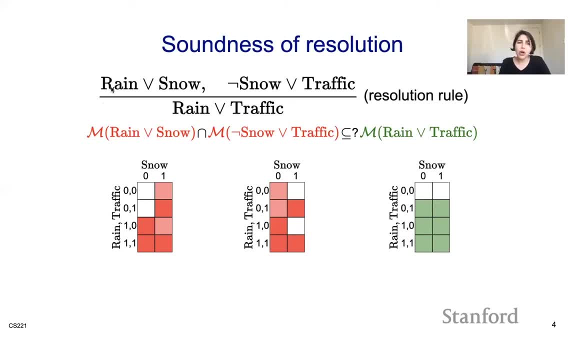 and I need to check entailments, So let's check that on this example. So if I have rain or snow, what is models of rain or snow, Models of? so I have here my truth table is going to be a little bit larger because I have 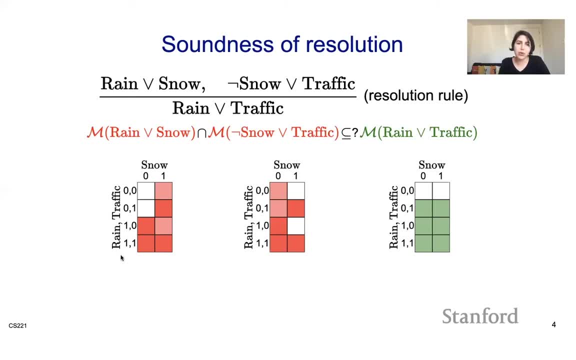 both snow, rain and traffic. So I need to look at zero one values for all of them. So I have rain or snow. Rain or snow correspond to these shaded areas, So that's models of rain or snow. And then I have models of not snow or traffic. that corresponds to these shaded areas And remember. 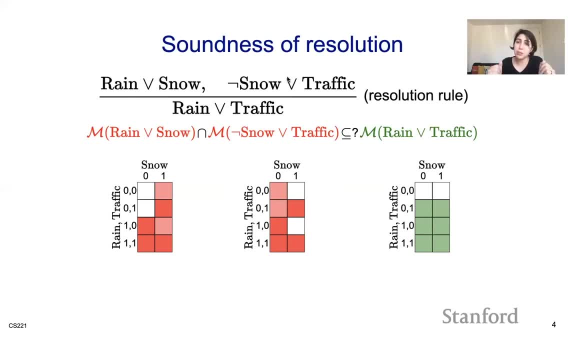 as I add more formulas to my knowledge base, I'm shrinking its models. I'm adding more constraints, so I'm shrinking the models. That is why models of these two formulas is going to be the intersection of their models. So the intersection is going to be this darker red area. So if I'm checking, 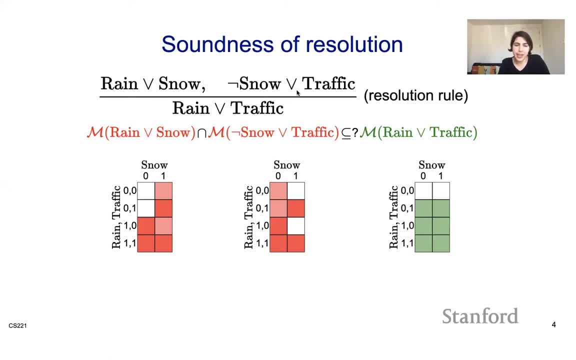 entailment. if I'm basically checking if resolution is sound, I should be checking entailment, And what that means is I should be checking if the models of what is in my knowledge base is going to be a subset of models of this new formula that I'm trying to derive here. So what's the new formula? 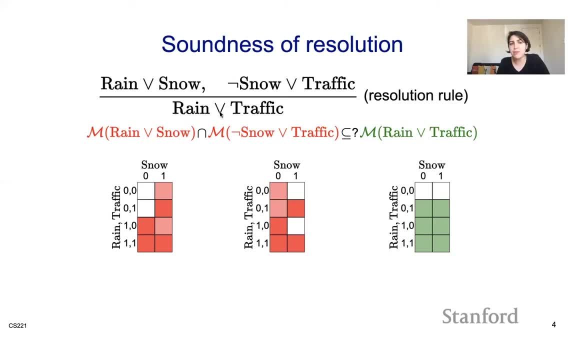 I'm trying to derive here. Resolution tells me you can derive rain or traffic, And if I look at rain or traffic and models of rain or traffic, I get this green area. So the question is: is the shaded dark red area a subset of the green area? And in this case it is. So it turns out that the 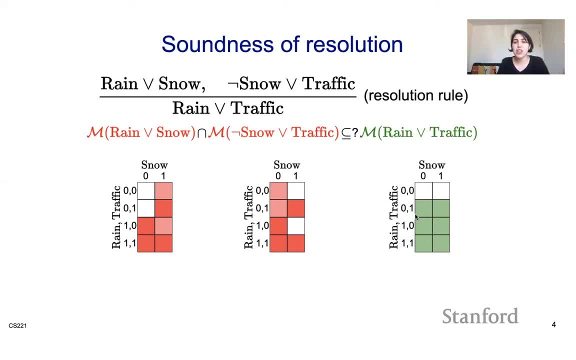 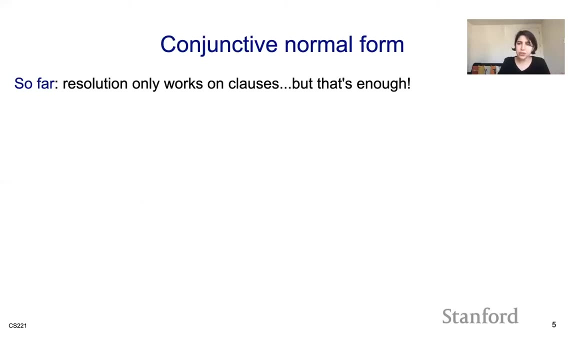 resolution is actually sound. So, in terms of thinking about the models, the models, the models, thinking about the semantics, here we are getting soundness, We are ensuring that we are getting truth by applying resolution. So resolution is sound. So, as you've seen, resolution only works on clauses. 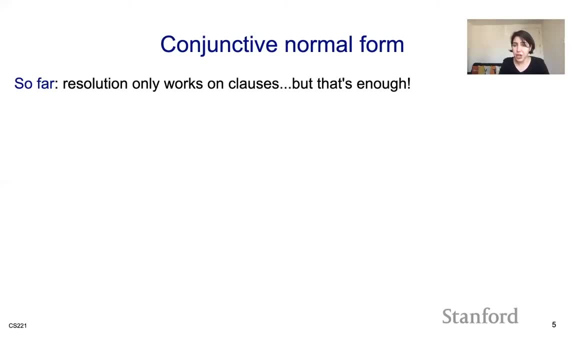 I've been defining these clauses, which are disjunctions of literals, And the question is: can I apply resolution to all of propositional logic? And the answer is yes. It actually turns out that the fact, because if resolution only works on clauses, that is actually enough. 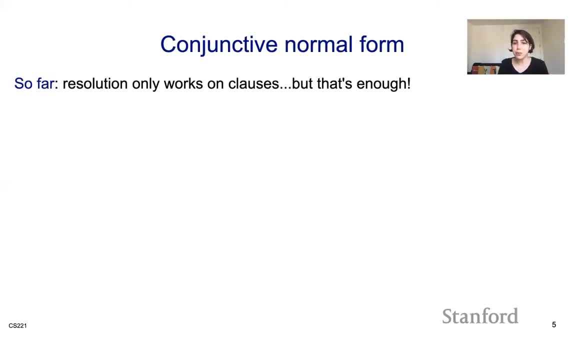 And the reason that is actually enough is you can think about any propositional formula And you can write any propositional formula as a conjunction of a bunch of clauses And that's called a conjunctive normal form. So a conjunctive normal form, a CNF formula, 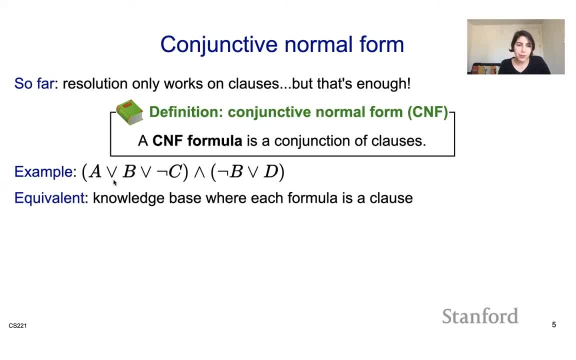 is a conjunction of clauses. So an example of that is: you have a clause A or B or a negation of C. You have another clause, negation of C, You have negation of B or D And an AND of these two clauses. 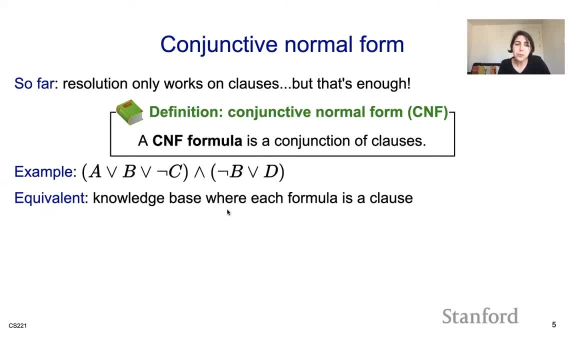 is in a conjunctive, normal form. So you can think of this as the equivalent of having a knowledge base where you have each formula is a clause And when you have a bunch of formulas in your knowledge base, you're basically thinking about AND of those formulas. 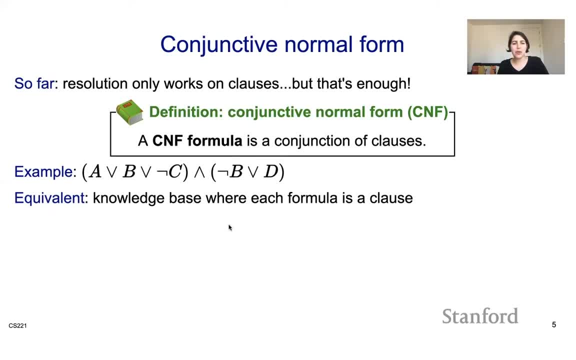 So a knowledge base basically is an AND of a bunch, of a conjunction of a bunch of formulas that could be written, let's say, as clauses. All right, So then basically every formula that is written in propositional logic can be converted into a conjunctive, normal form. 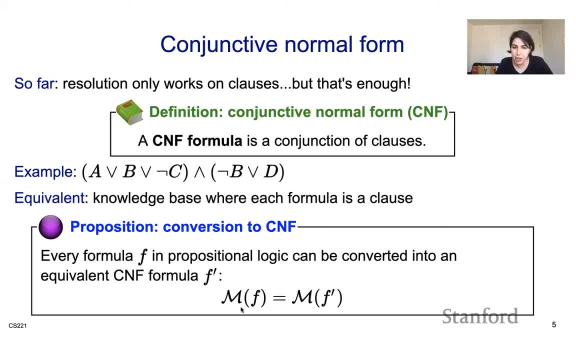 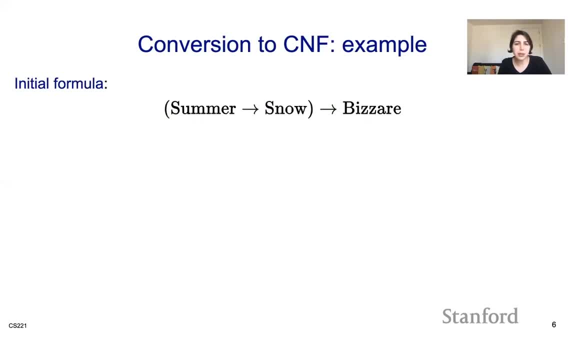 in a new formula conjunctive normal form. that's exactly equal, like the models of the old formula is exactly equal to the models of the new formula. So how can we do that? It's actually a kind of easy way of doing it. 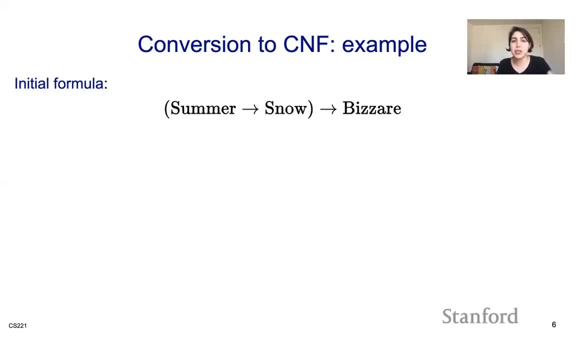 There's just a recipe for converting every formula to conjunctive. Let's look at an example. So let's say that you have a formula It says summer implies snow and the whole thing implies bizarre. So here I don't have any ANDs or ORs. 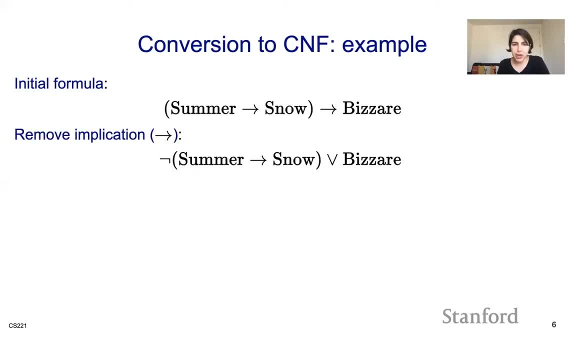 I have this implication, So I need to get rid of that implication. How can I do that? I can basically remove implication and write it out in the form that I talked about earlier, which is negation of the first term or the second term. 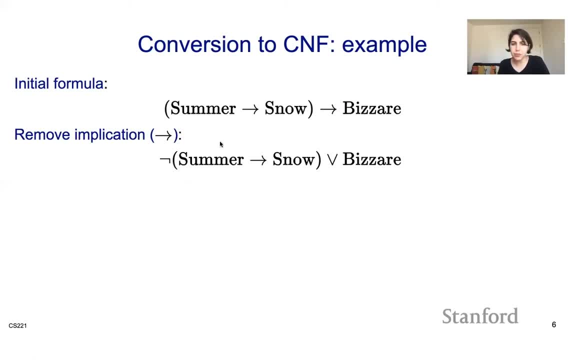 So this implication, I can write it as negation of the first term, This whole term or the second term. I can remove this implication and write it in a similar way. I can write it as negation of summer or snow. So now what I'm going to do is I'm 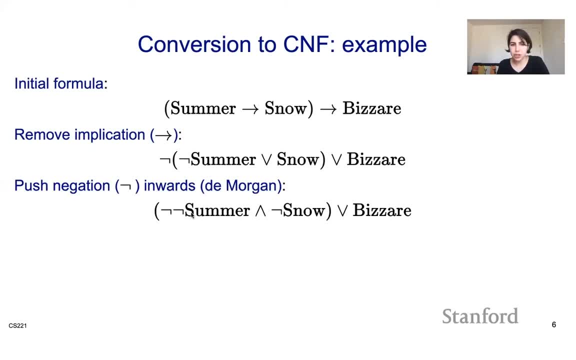 going to push the negation inside using the Morgan's law. So I'm going to push the negation inside. make this AND push the negation inside. I have a double negation here. I'm going to get rid of that double negation. 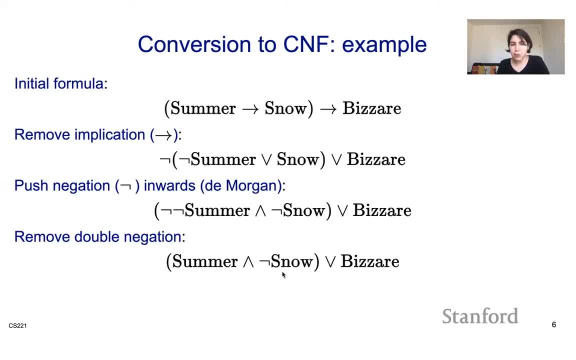 and make this positive. So now I have a bunch of literals, positive or negative, And I only have ANDs and ORs. but this is actually not in the conjunctive normal form, Because conjunctive normal form means that AND of a bunch of ORs. this is actually the opposite. 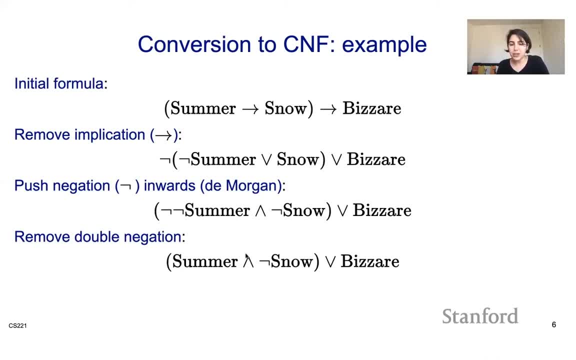 This is OR of a bunch of ANDs, But you can actually distribute this OR over the AND And then you end up, if you distribute the OR over the AND, you end up with these two clauses: summer, or bizarre, and another clause which is negation of snow, or bizarre. 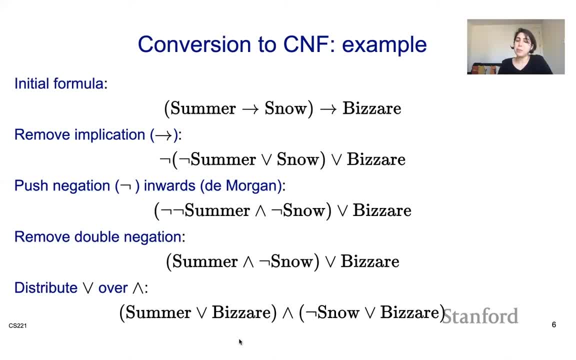 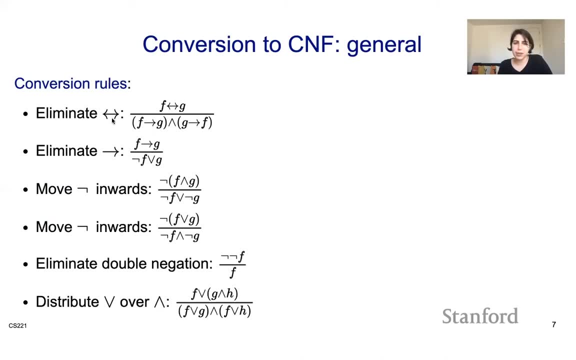 So you end up in a CNF form. Any formula you give me, I can end up in a CNF form. So the general recipe for it is: if you have implications or these bidirectional implications, replace them with ANDs and ORs and negations. 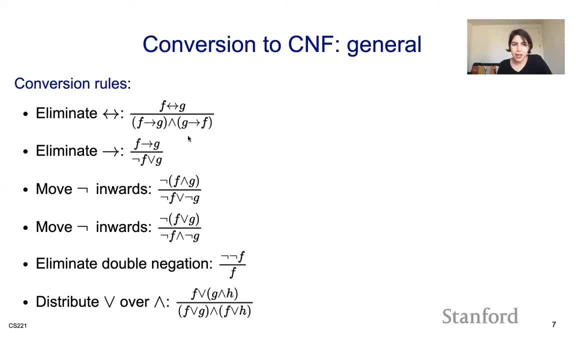 So that's the first thing you want to do: Bidirectional implication: write it out as implications and ANDs. If you see an implication, write it out as a form of negation. and OR. If you have any negations, move them. 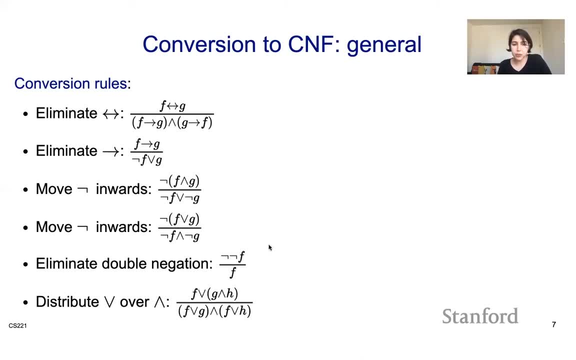 inside, using the Morgan's law, If you have double negations, remove the double negations And then at the end just distribute OR over, AND if you have anything of that form And you'll end up with a conjunctive, normal form. 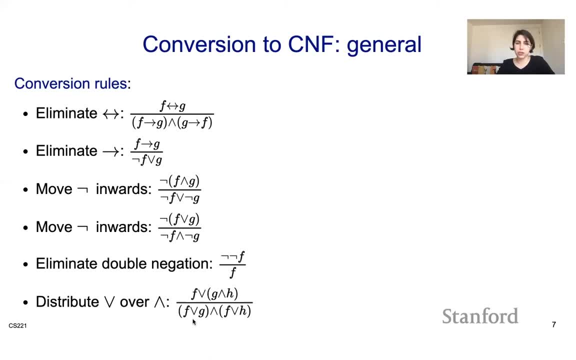 So that is kind of the general recipe of converting any propositional logic formula to a CNF form. And then why are we writing this as a CNF form? Because the resolution rule works only on clauses, which only works on CNF form formulas. 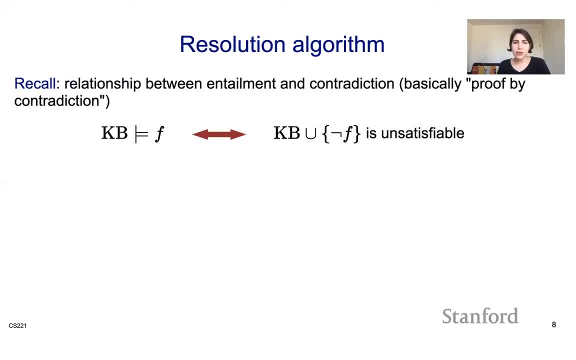 All right. So what's the idea of resolution algorithm? Well, why are we trying to run resolution? The reason is, in general- you might be asking me if F is true or not- We care about having that assistant that we can ask from. 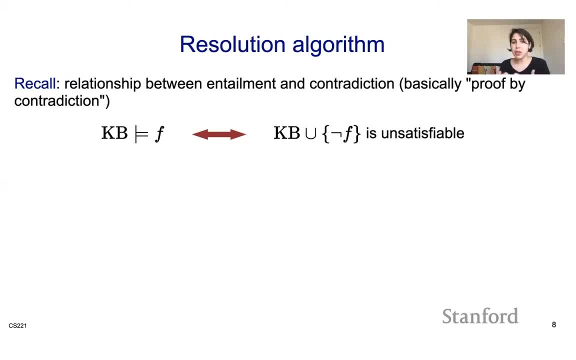 or we can tell it things, And what does that do? That tries to basically check things like entailment. So if the knowledge base, if you want to check if the knowledge base is entailing a new formula or not, that's the same thing. 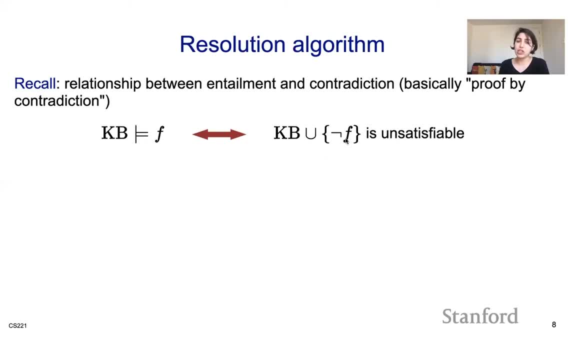 That's the same thing as checking if negation of F, if the knowledge base contradicts negation of F, or basically checking if negation of F added to the knowledge base is unsatisfiable or not. So how do we run the resolution based algorithm? 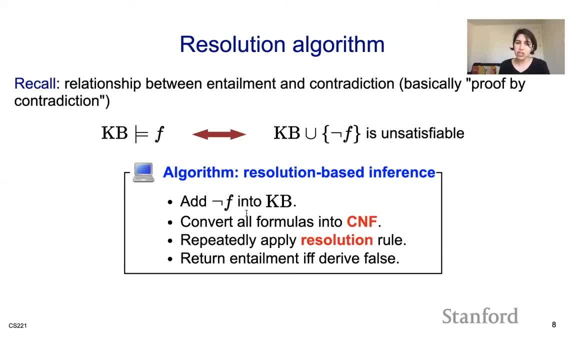 Well, what we do is, if you ask me if F is entailed or not, I'll add negation of F to my knowledge base, And then I convert all my formulas to CNF form. We can do that, And once I have everything in a CNF form, 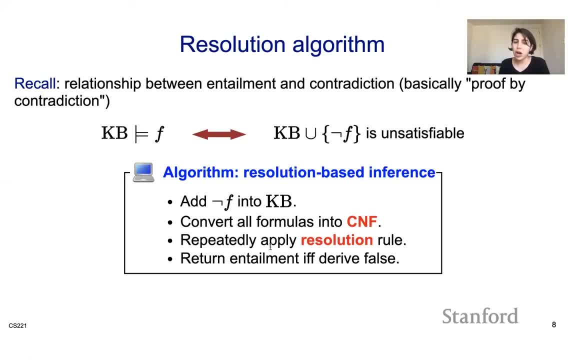 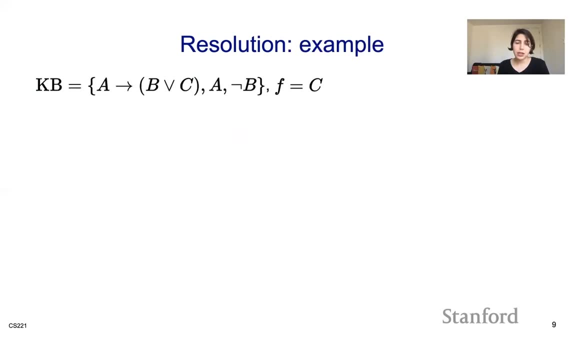 I can apply a resolution. I can keep repeatedly applying resolution until everything is converged And then I can return entailment, even only if I'm deriving false. So that is how we run resolution. if we want to answer a question about entailment, Let's look at an example here. 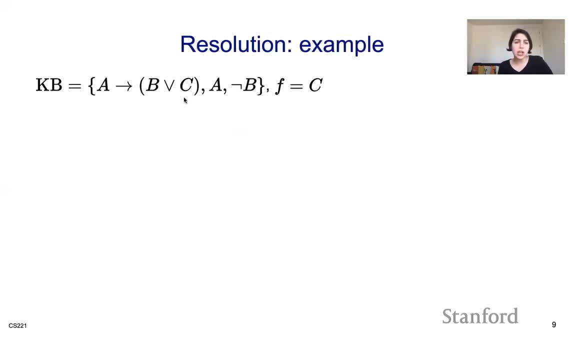 So let's say I have a knowledge base. This is my knowledge base. It has a bunch of things in it. They're not in a CNF form, They're not in a clause form or anything, But I have a bunch of formulas. 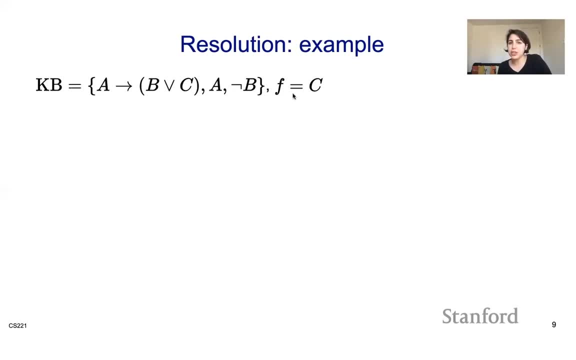 And you're asking me if this knowledge base entails a new formula, and that new formula is C. So how do I check that using resolution? What I'm going to do is I'm going to add a negation of C to my knowledge base. 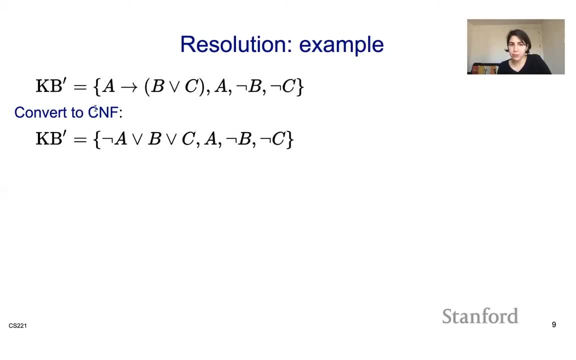 I'm going to make sure that I'm not going to have a problem. I'm going to make everything to a CNF form. so using that recipe that I talked about removing implications and pushing negations in and distributing ors over things. 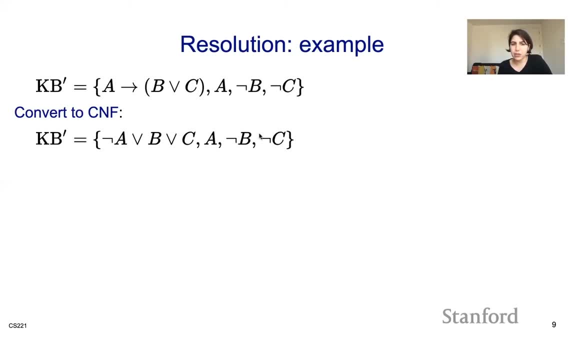 Once I do that, everything is in a clause form. I have a clause and I have literals. So this is my knowledge base: Everything is in the clause form, in a CNF form, And then I'm going to repeatedly apply a resolution. 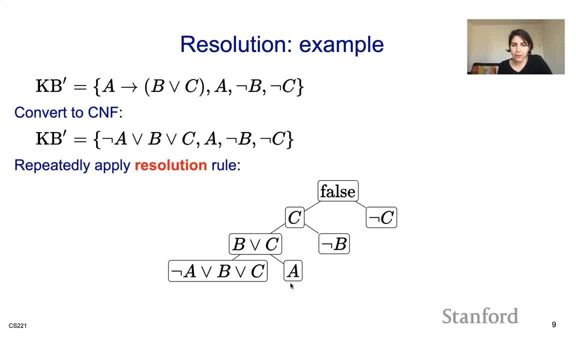 So how do I apply resolution? Let's start from these two. So I have A and I have negation of A or B or C. In some sense, A and negation of A gets canceled out, So I can add B or C to my knowledge base. 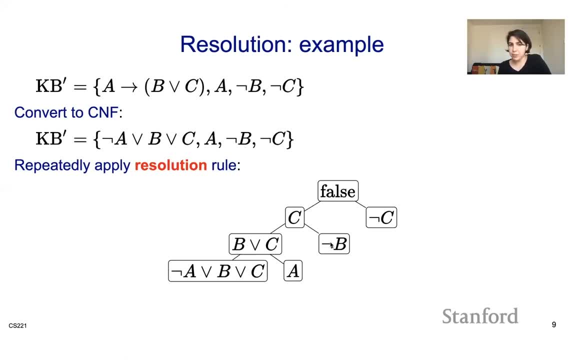 using resolution. I have negation of B in my knowledge base, So negation of B and B get canceled out And I can add C to my knowledge base. And I've added negation of C to my knowledge base And negation of C and C get canceled out and I'll get false. 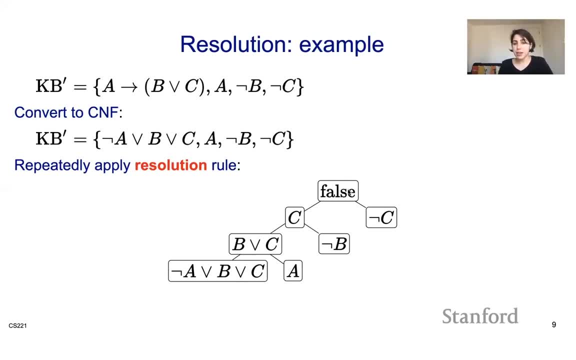 So, after repeatedly applying resolution here, I'm getting false meaning that when I add negation, I'm going to get false. So I'm going to get false meaning that when I add negation of the formula. I was able to get this contradiction. 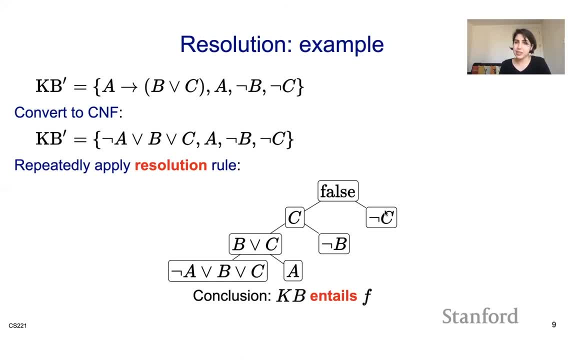 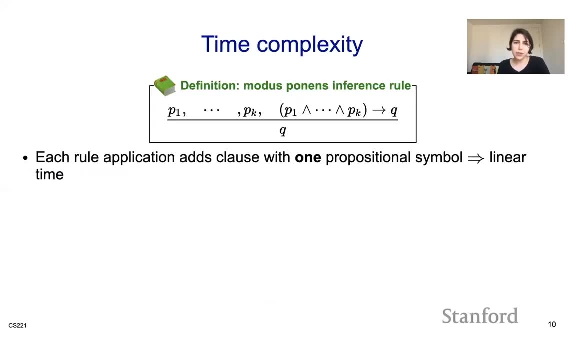 I was able to get false, And what that means is that knowledge base actually entails the formula, the formula being C in this case. So knowledge base entails C. I can derive C All right. so a good question to ask is: what is the time? complexity of these algorithms. 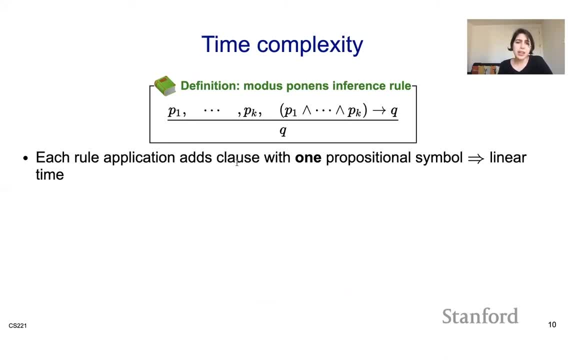 So, if you remember modus ponens, the idea of modus ponens- this was the more general form of it- was that at every step, you have to add one propositional symbol to our knowledge base. And if you're adding one propositional symbol, 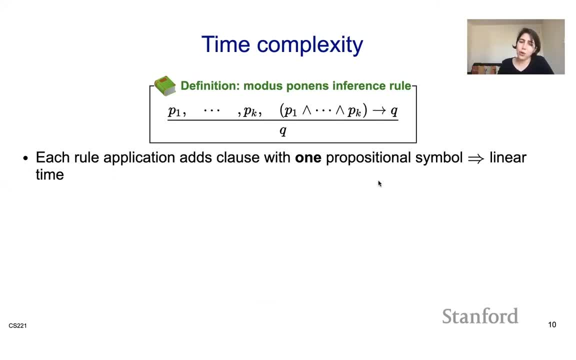 if you have n of them, you have at most n things to go over. So this would be a linear time algorithm. when you're running modus ponens, It's pretty simple. It also converges fairly quickly because there are n things that we need to go over.